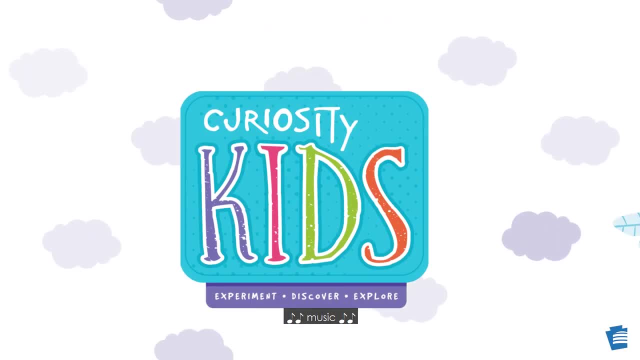 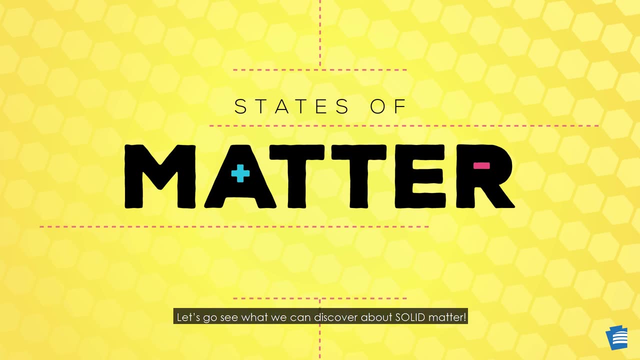 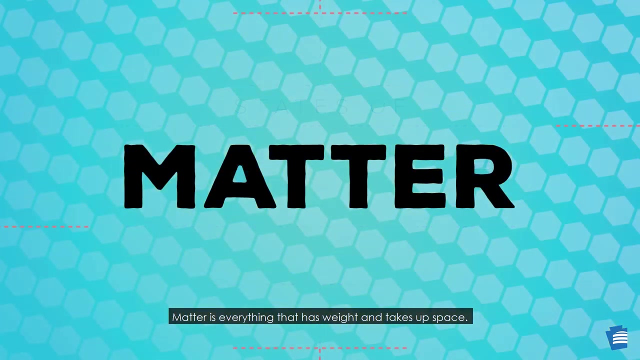 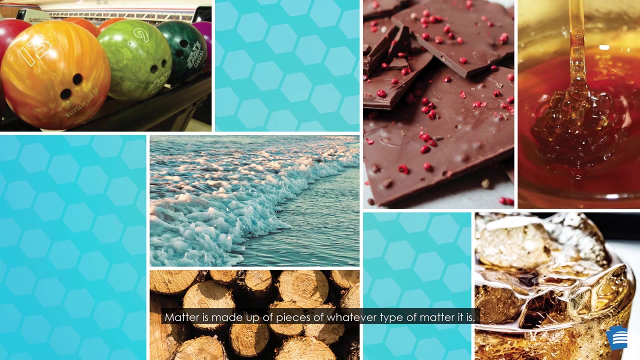 Hello Curiosity Kids. Do you know what matter is? Let's go see what we can discover about solid matter. Matter is everything that has weight and takes up space. Everything is made of matter, whether it's a solid, liquid or gas. Matter is made up of pieces of whatever type of matter it. 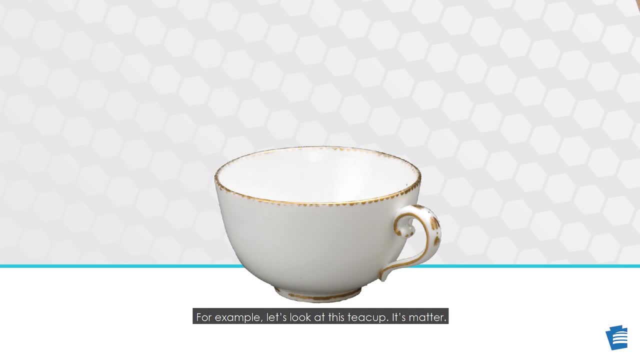 is, For example. let's look at this teacup. It's matter If I take a hammer and break it into pieces. it's still the same type of matter. It's still a teacup, just in smaller pieces. 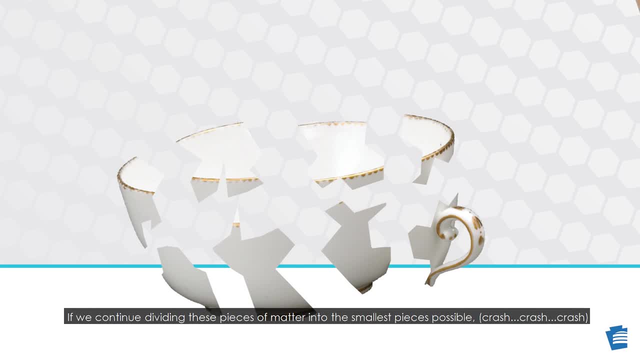 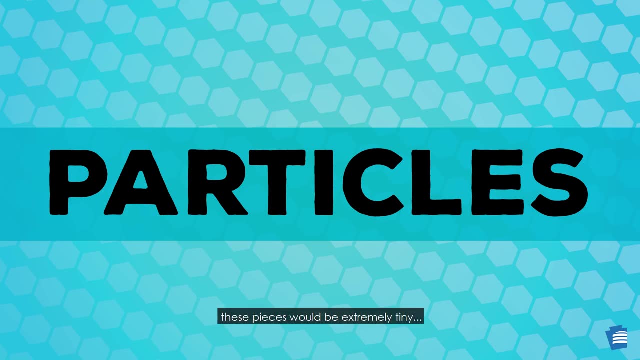 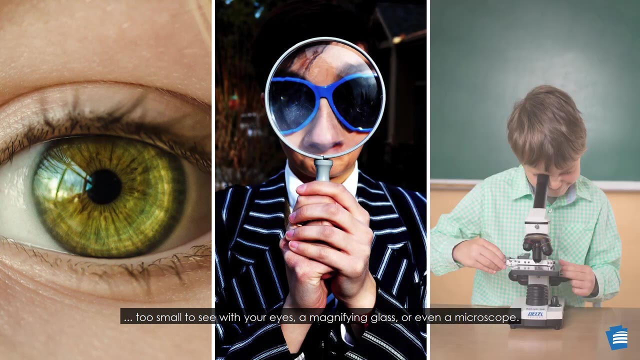 If we continue dividing these pieces of matter into the smallest pieces possible, called particles, these pieces would be extremely tiny, too small to see with your eyes- a magnifying glass or even a microscope, Even though we can't see these particles. 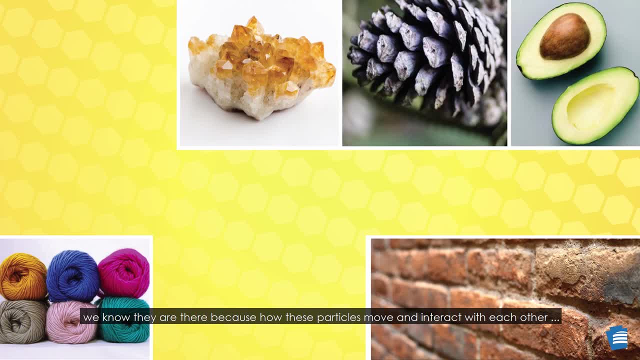 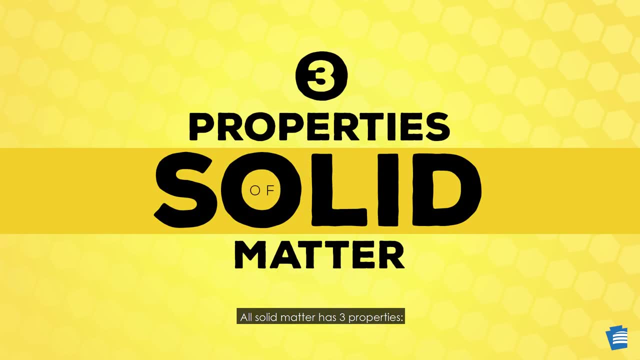 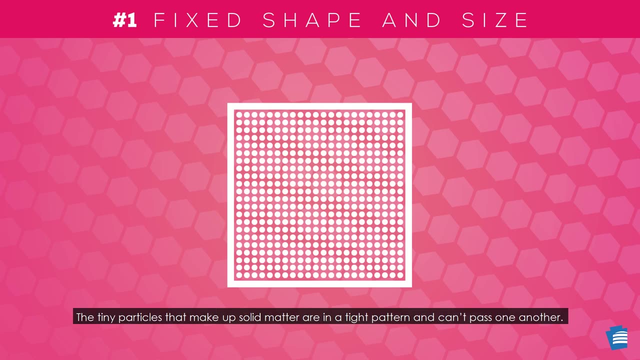 we know they are there because how these particles move and interact with each other explains what makes matter a solid. All solid matter has three properties. Solid matter has a fixed size and shape. The tiny particles that make up solid matter are in a tight pattern and can't. 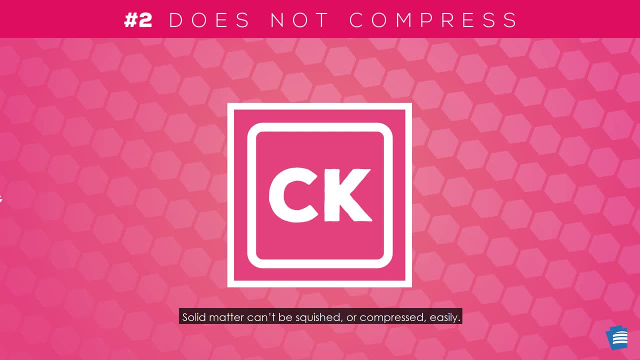 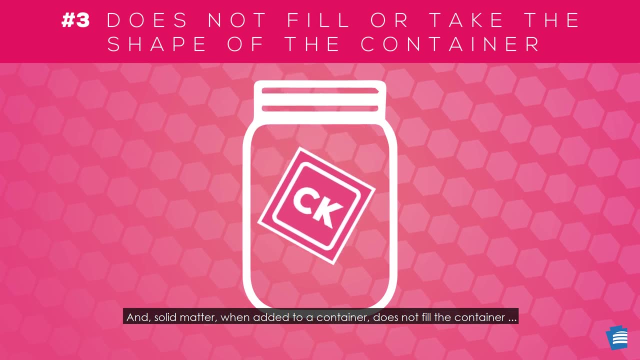 pass one another. Solid matter can't be squished or compressed easily, And solid matter when added to a container doesn't fit. Solid matter can't be squished or compressed easily. Solid matter when added to a container doesn't fit. Solid matter can't be squished or compressed easily. Solid. 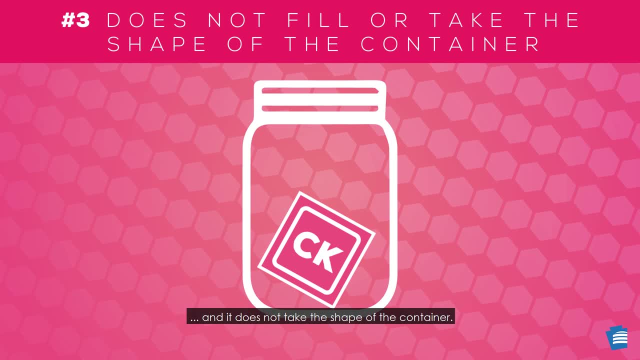 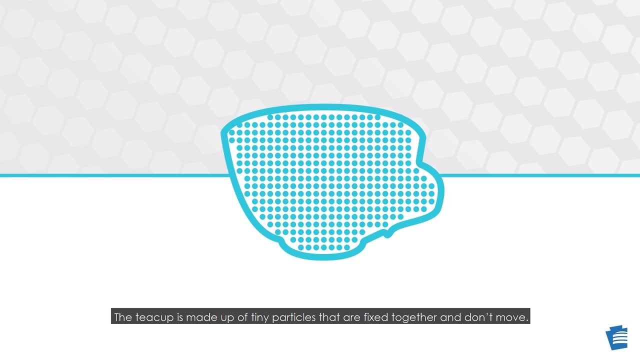 matter, when added to a container, doesn't fit. Solid matter can't be squished or compressed easily And it doesn't take the shape of the container. Let's look at my teacup again: It is solid matter. The teacup is made up of tiny particles that are fixed together and don't move. Teacups don't. 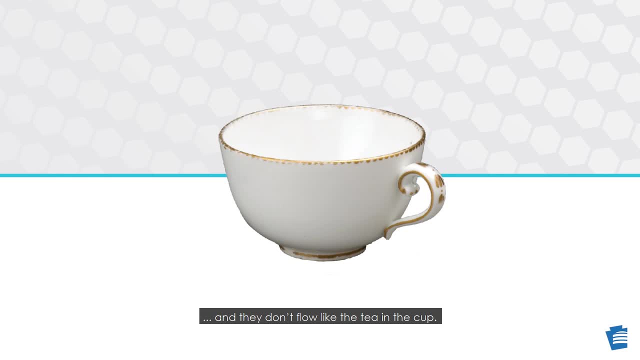 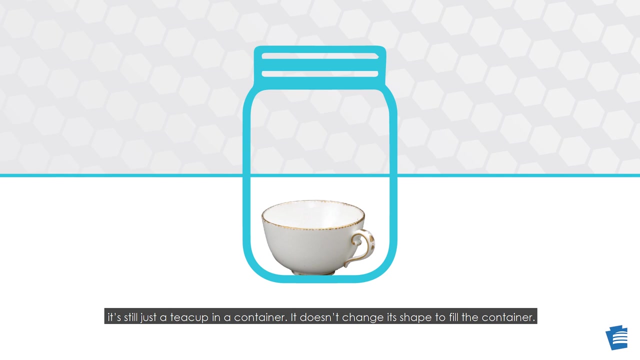 change shape. Teacups aren't squishy and they don't flow like the tea in the cup. If I put the teacup into a container, It's still a teacup in a container. It doesn't change its shape to fill the container.